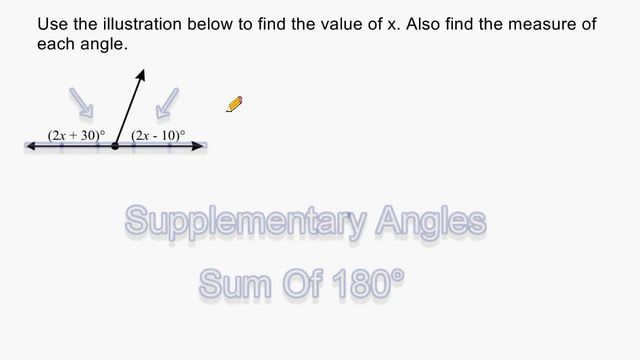 going to use this information to figure out what the value of x is. On the left, we have an expression that reads 2x plus 30, and on the right, we have an expression that reads 2x minus 10.. Because we know that both angles have a sum of 180 degrees, we are going to 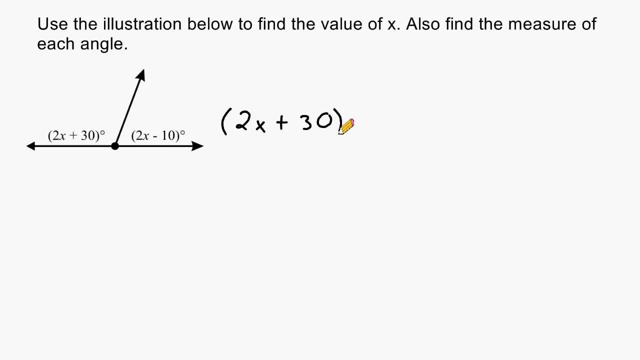 take 2x plus 30 and add that to 2x minus 10 and set that equal to 180 degrees, And then all we have to do is figure out what the value of x is by isolating that variable. Now, right below I am going to write 2x plus 30 and because we have a plus sign, we can. 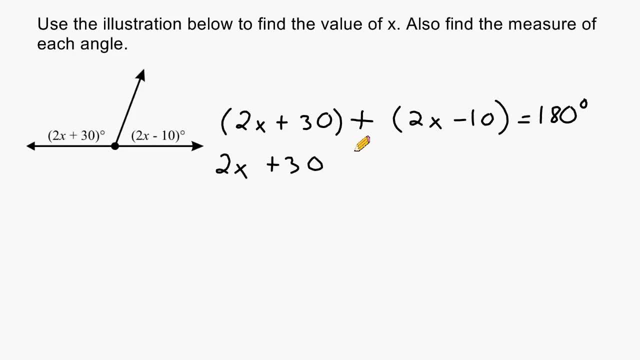 keep every term inside the next set of parentheses the same. When there is only a single plus on the outside of parentheses- remember there is really a number 1 there- It is like saying positive 1, so we could distribute a positive 1 to each term inside parentheses. essentially, 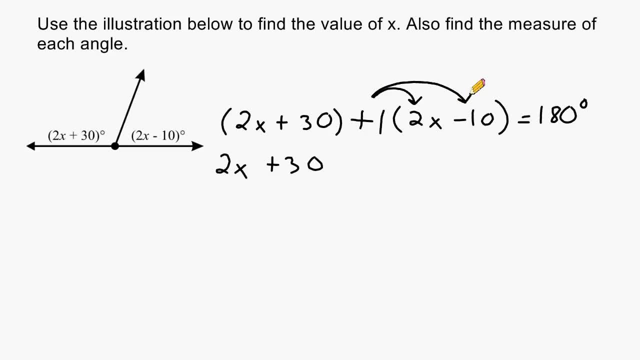 keeping each term the same. If there was a minus sign, we would have to multiply negative 1 by each term inside parentheses. So 1 times 2x is 2x and 1 times negative 10 is negative 10.. And this whole expression. 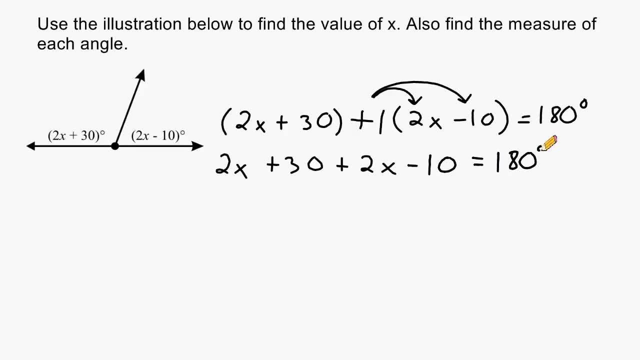 is still equal to 180 degrees. The next thing that we are going to do is combine like terms, So we can combine the 2x to this 2x, giving us a sum of 4x, And then we can combine the 30 with the minus 10.. 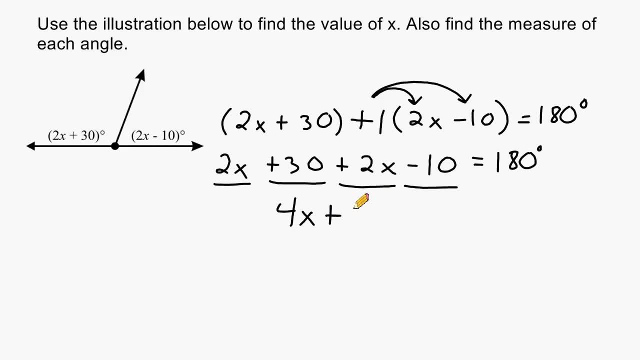 And 30 minus 10 is a total of 20.. So now we have the equation: 4x plus 20 is equal to 180 degrees. The next thing that we have to do is isolate our variable. So we are going to start by. 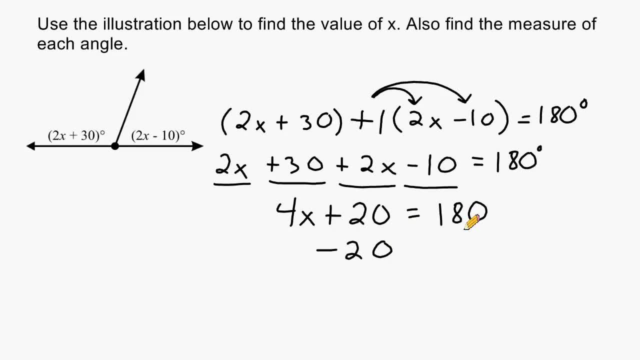 subtracting 20 on the left and moving it over to the right side of our equation, And we have to do the same thing on the right that we did on the left, So we balance out our equation. So on the left, all we have remaining is 4x, And on the right we have the same thing on. 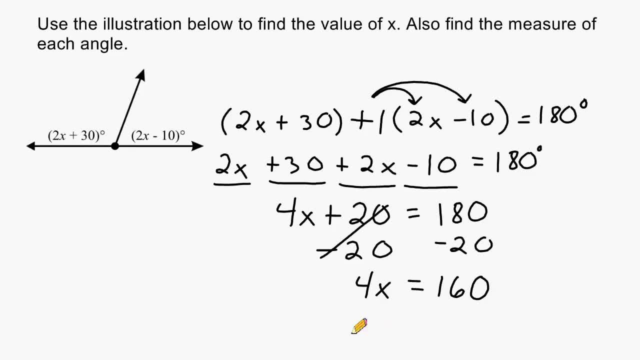 the left, We have a total of 160.. Because our goal is to have 1x at the end of our equation, we are going to take the number 4 and divide it by itself, because anything divided by itself is one whole And we have to balance our equation, so we have to also divide the other side by